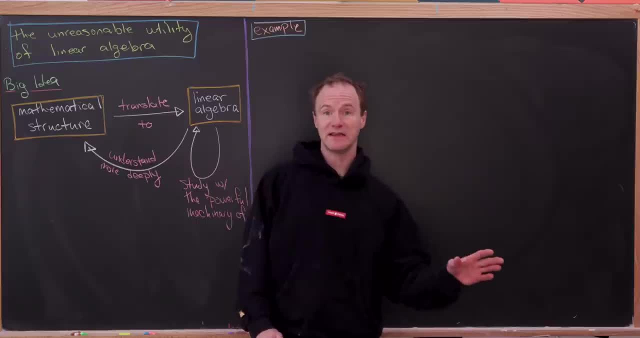 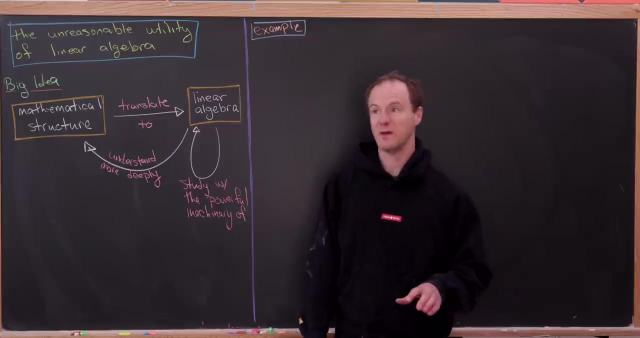 that is how we can explore some ideas that don't seem connected to linear algebra, via linear algebra. So what's the big idea here? Well, you want to start with a mathematical structure. You know, maybe that's going to be a group, or maybe that's going to be some. 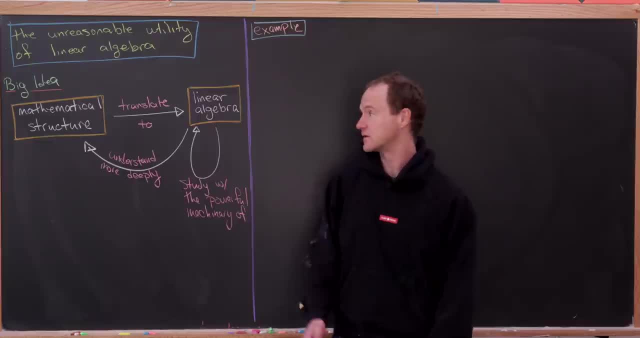 sort of algebraic structure or maybe that's going to be the derivative or something, And then you want to translate that mathematical structure into the language of linear algebra And once you're in this linear algebraic setting, you can study this setup with the powerful. 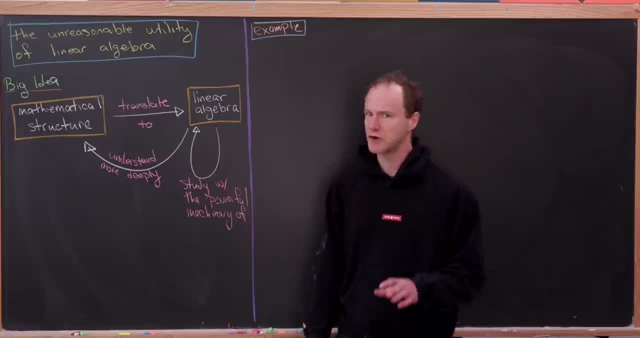 tools that you have, The tools of linear algebra, And so there are many, many powerful tools of linear algebra. We'll see some of them, And while studying inside of this linear algebra framework, you get more deep understanding of the original mathematical structure. 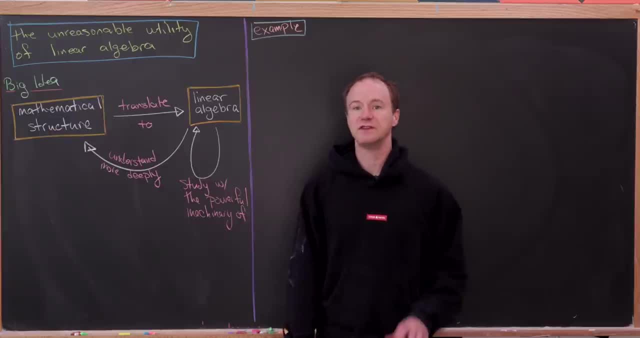 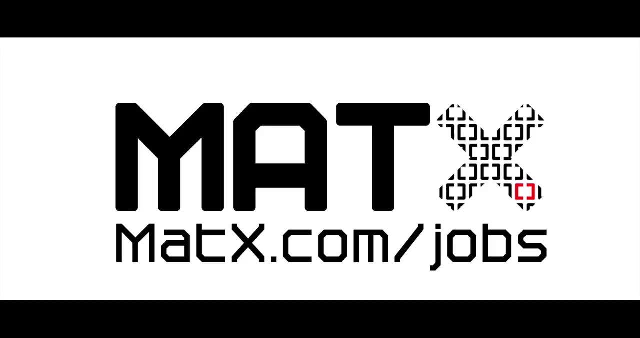 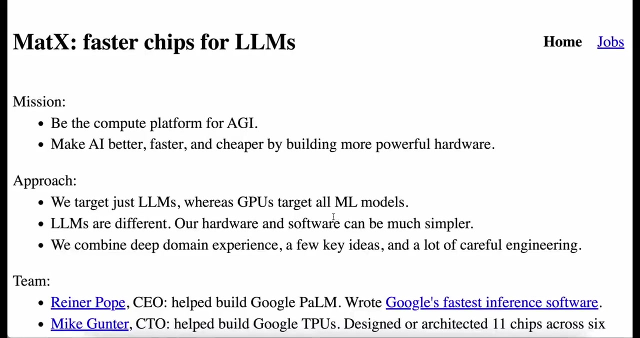 Okay, so now that we have an overview of what we want to do today, let's jump into our first example. I'm really excited to tell you about the sponsor for today's video. Instead of like normal linear algebra, we're going to talk about a company called MatX. MatX is a company developing 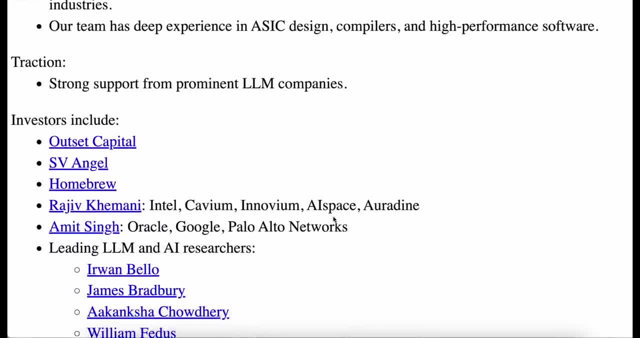 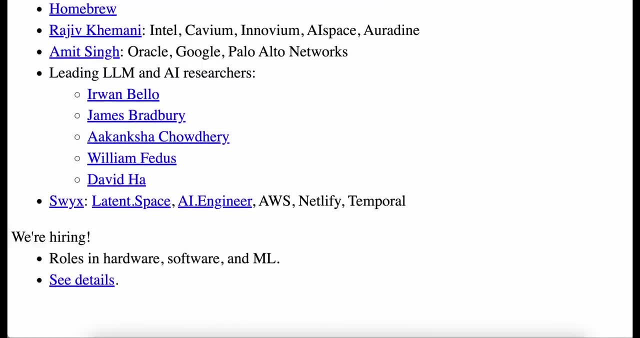 chips for large language models. By investing all of their silicon in this specialized application, their chip can perform much better than GPUs And they're hiring software compiler, machine learning and silicon engineering roles And I think probably most of you are familiar with. 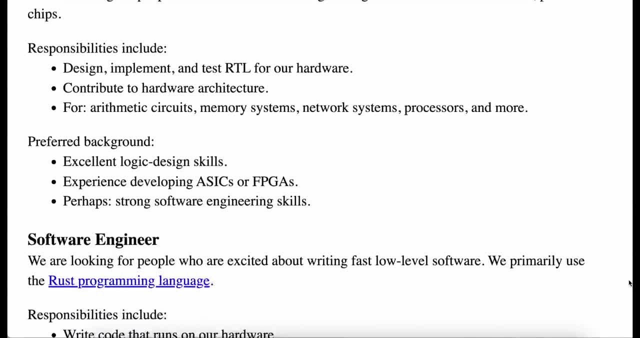 MatX. MatX is a software compiler, machine learning and silicon engineering role And I think probably most of you are familiar with MatX. MatX is a software compiler machine teamwork And I think probably there are many, many people out there in the audience. 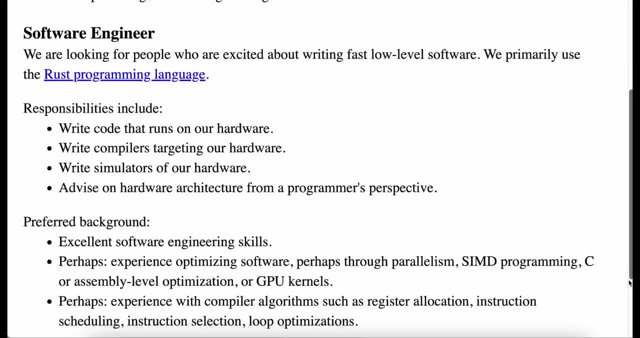 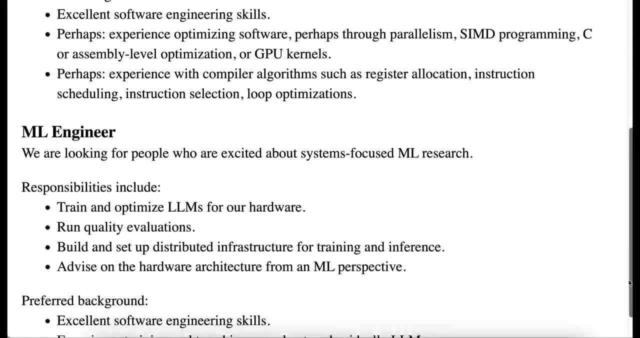 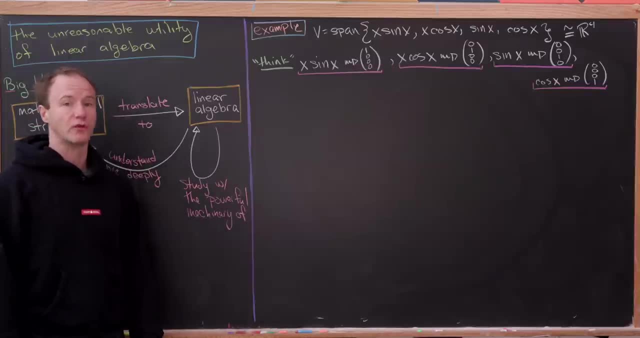 that would be perfect for this type of position. So head over to matxcom cannonball for more information and to apply if you're interested. Thanks once again to MatX for sponsoring today's video. So for our first setup, let's consider a four dimensional real vector space. I'll call it V. 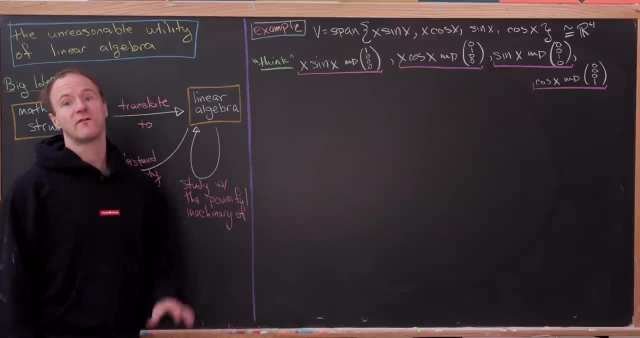 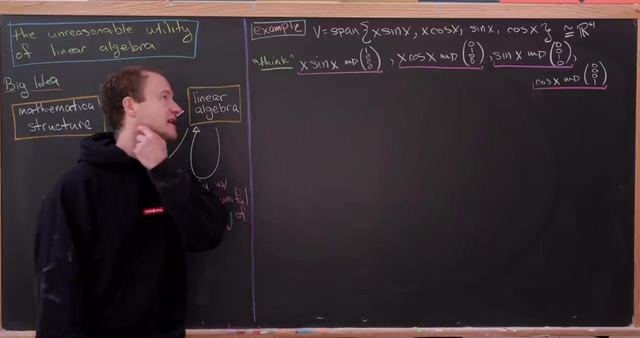 And I'm going to span it by the following four functions. So let's recall, the space of smooth functions makes a vector space and this is simply a subspace of that larger vector space. So my four functions are x times sine x, x times cosine of x, sine x and cosine of x. 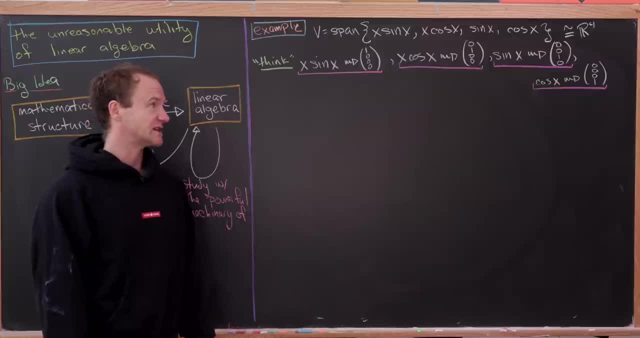 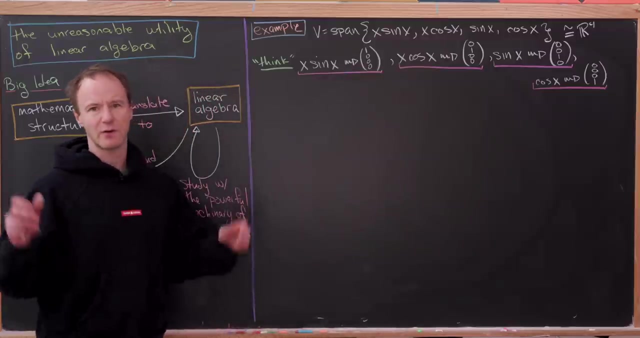 But since this is four-dimensional, it has four basis vectors. that means it's isomorphic to R4, where we think of that as just four-entry column vectors, And that isomorphism can be given by the following rule: that this is how we want to think about it. 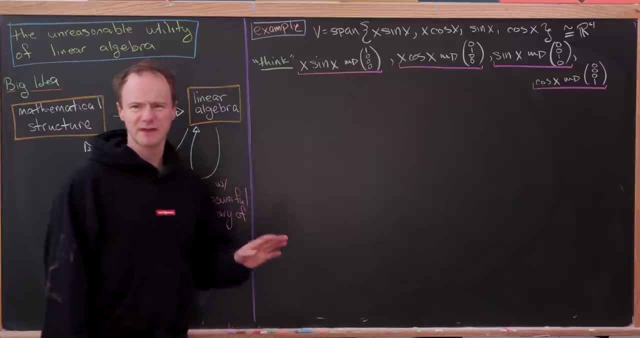 So x sine x is assigned to well, sometimes that's called the vector E1, so it's 1, 0, 0, 0.. Then x, cosine of x, is the next standard basis vector: 0, 1, 0, 0. 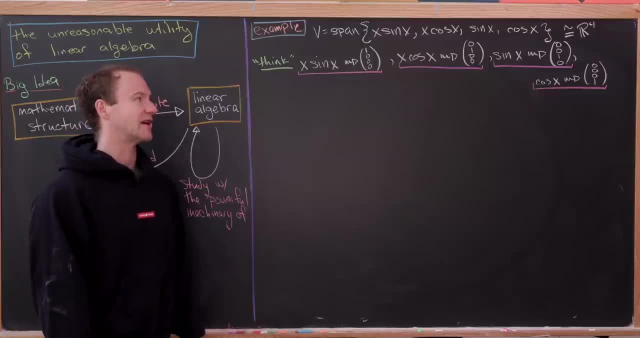 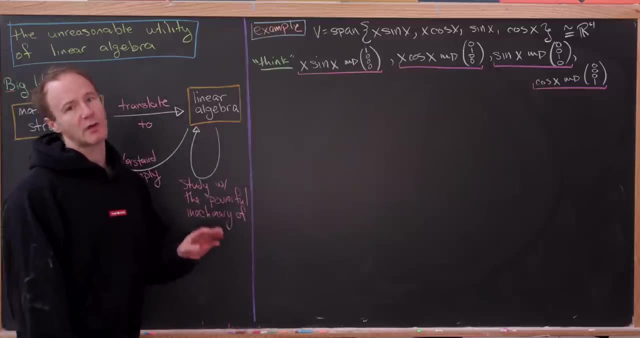 Sine x will assign to 0, 0, 1, 0.. And finally, cosine x will assign to 0, 0, 0, 1.. And what we want to do here? well, there are a number of things we could do. 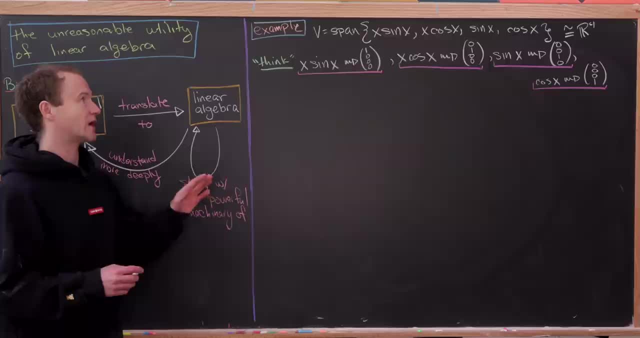 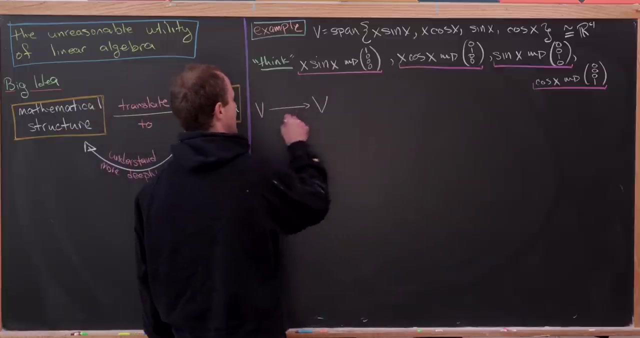 but let's just see what the derivative does to our space V and if we can turn that into a more familiar linear algebraic setup which might involve a matrix. Okay, so let's maybe make a diagram first. Let's say we've got this map from V to V. 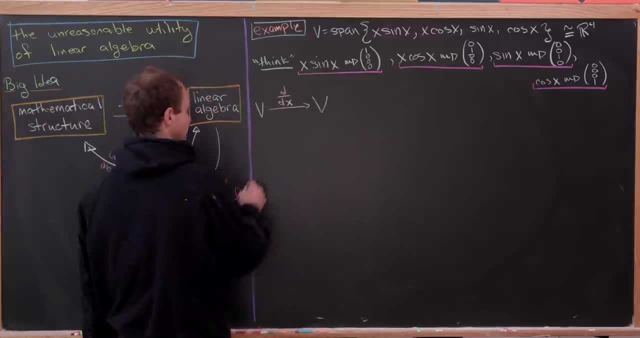 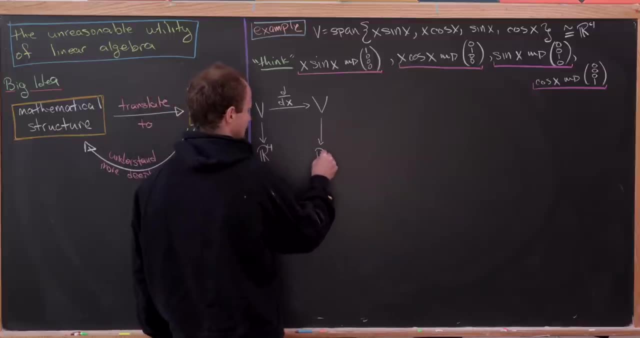 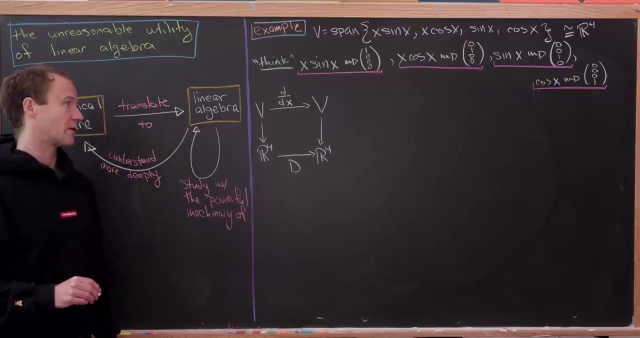 which is given by simply taking the derivative, And then we've got this assignment of V to R4 going down each of the sides, And then over here we've got something that I'll call capital D, which we'll see will be a 4 by 4 matrix. 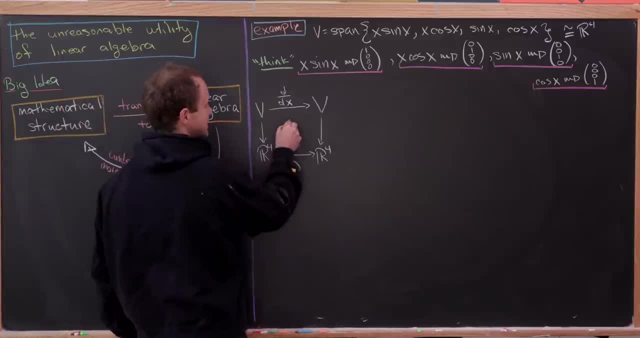 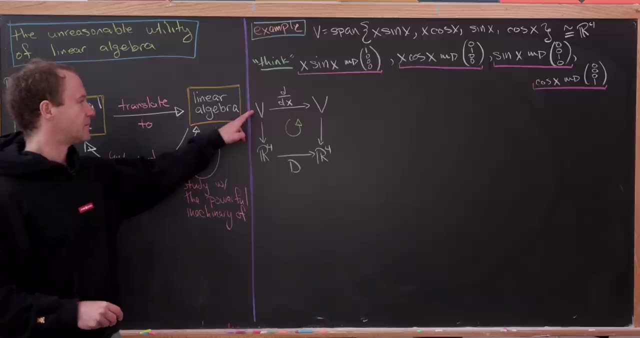 And we want to choose this, capital D, so that this is a so-called commutative diagram, which means we can start over here in capital V and take any path we want to R4 down here and we'll get the same result. 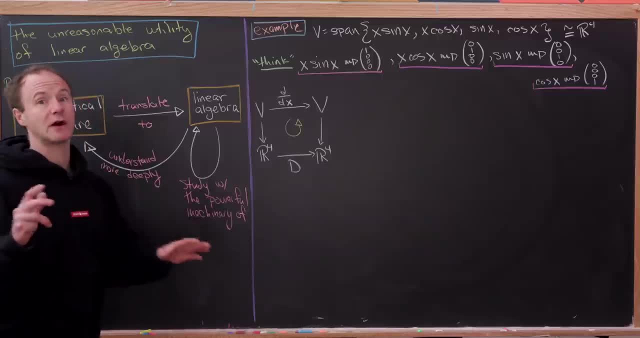 That means that in this setup, capital D will be a representation of our derivative. Okay, but let's recall, to get a matrix representation of any linear transformation, you really only need to know what it's doing to the basis vectors. So let's see that. 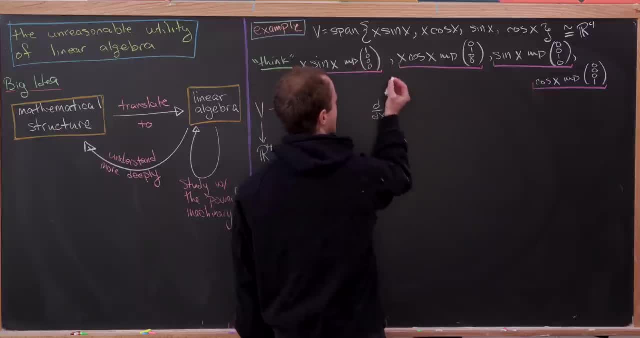 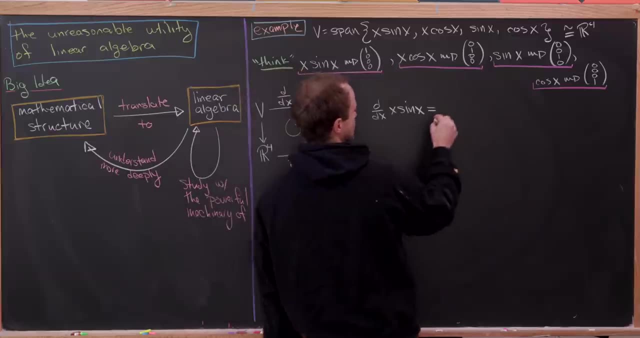 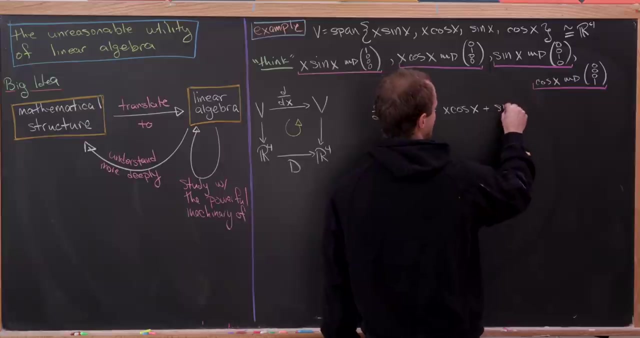 So we've got the derivative with respect to x of x. sine x equals what? Well, that's pretty easy. with the product rule. We'll have x times cosine of x and then plus sine of x. But then translating that into what we want this matrix to do, 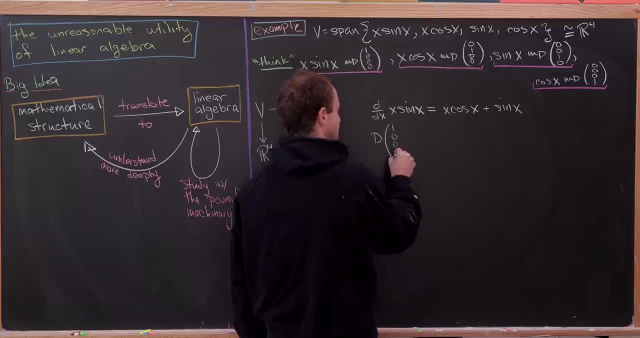 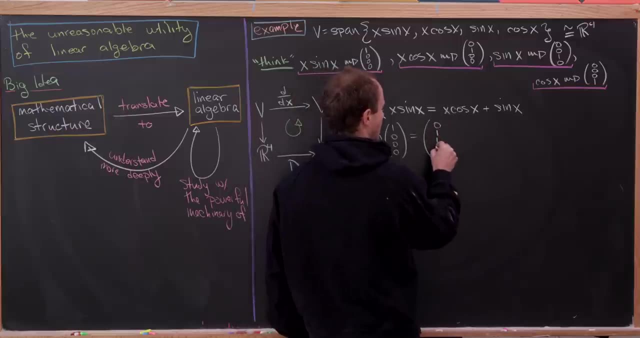 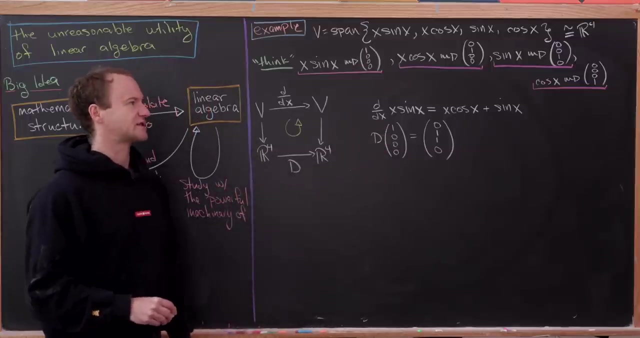 that means this matrix D should multiply into our vector 1, 0,, 0, 0, and give us the vector 0, 1, 1, 0.. That's because that's the vector of x sine x, and then the vector of x, cos x, plus sine of x. 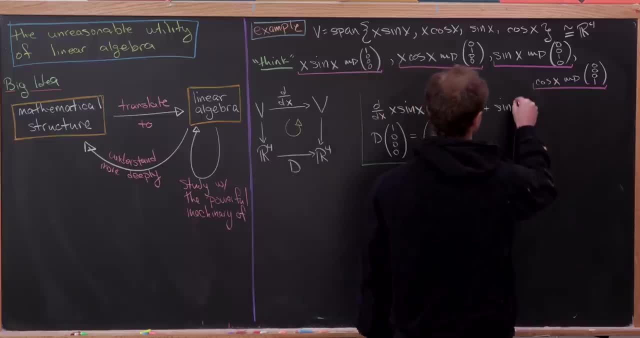 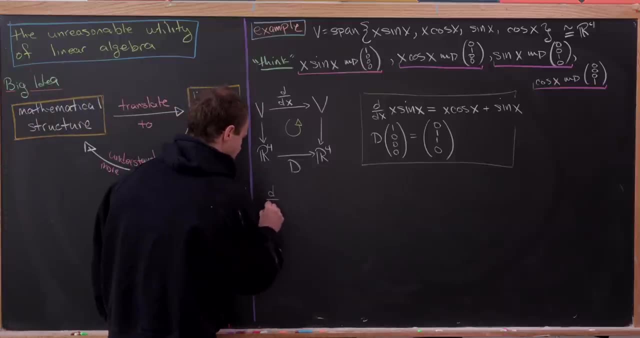 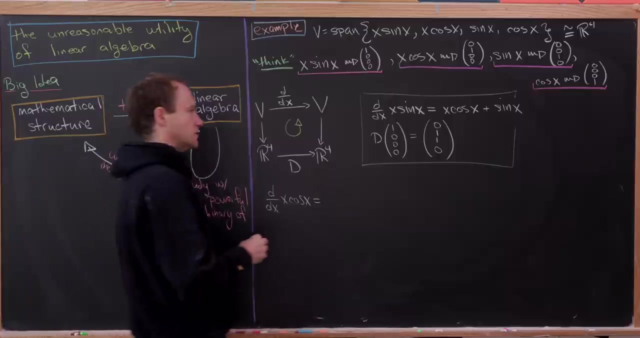 Okay, good. So this is giving us one idea of what's going on here with our matrix representation. Now let's look at another idea. So if we take the derivative with respect to x of x times cosine of x, again we can use the product rule. 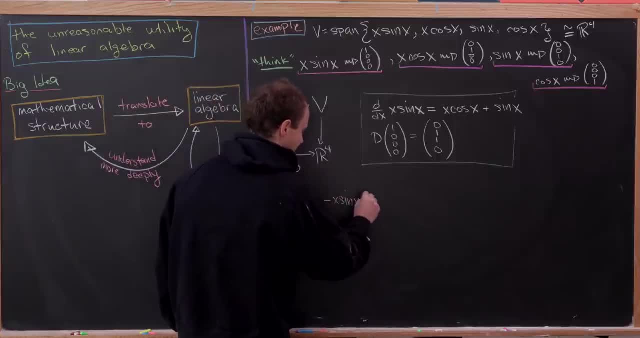 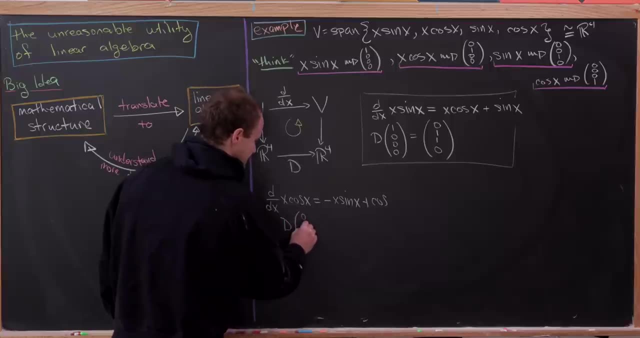 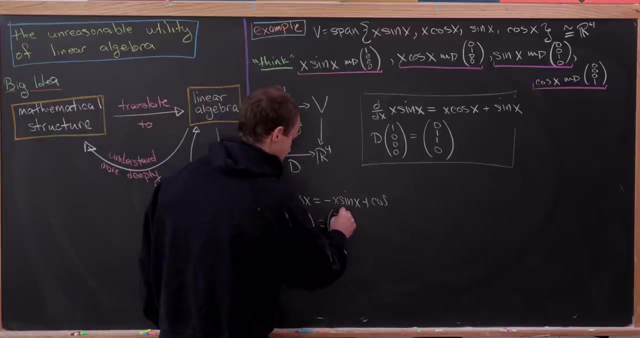 To give us minus x times sine x plus cosine of x. But if we turn this into a matrix vector setup, that means D should multiply into our vector E2, the second standard basis vector, and give us negative 1,, 0,, 0, 1.. 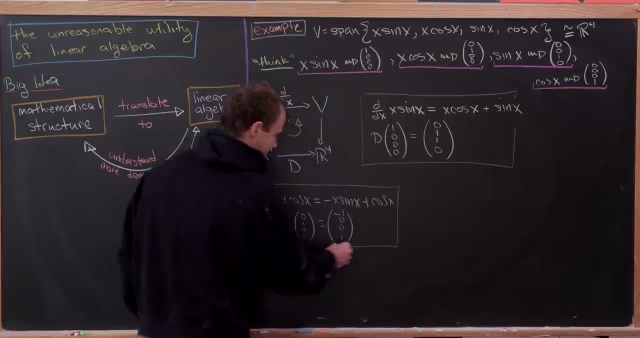 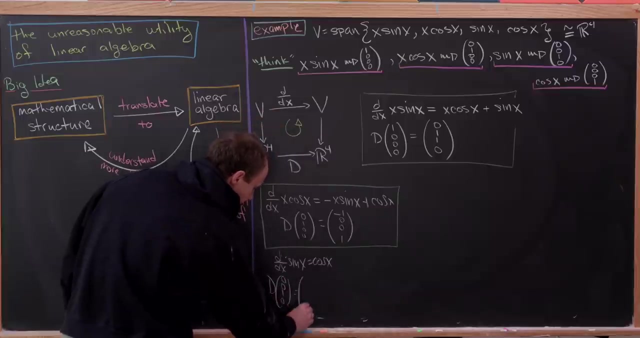 Okay, nice. Now let's see what happens to the remaining two vectors. So if we take the derivative with respect to x of sine of x, we simply get cosine of x, But that means D on the vector 0, 0, 1, 0 should give us 0, 0, 0, 1.. 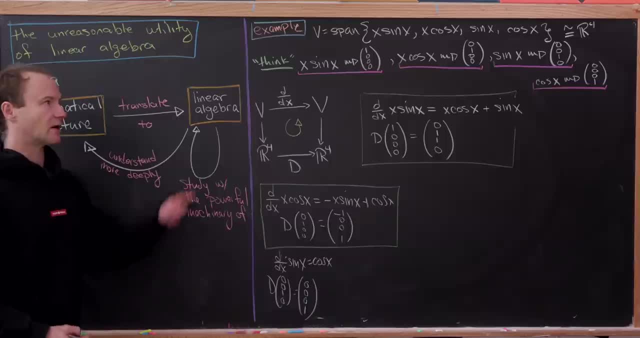 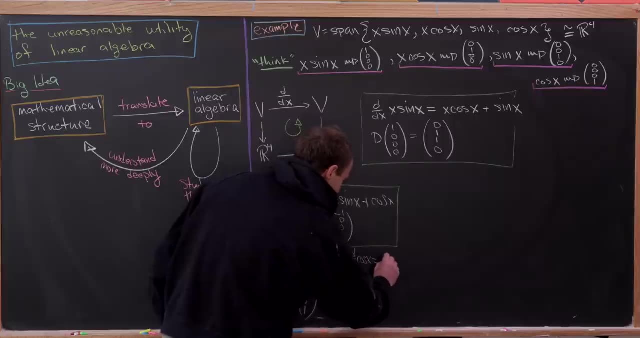 Just given the assignment that we're making throughout here, You know with the magenta underlines. And then finally, the derivative with respect to x, of cos. x is negative, sine of x, But that means D on 0, 0, 0, 1 should be 0, 0, negative 1, 0.. 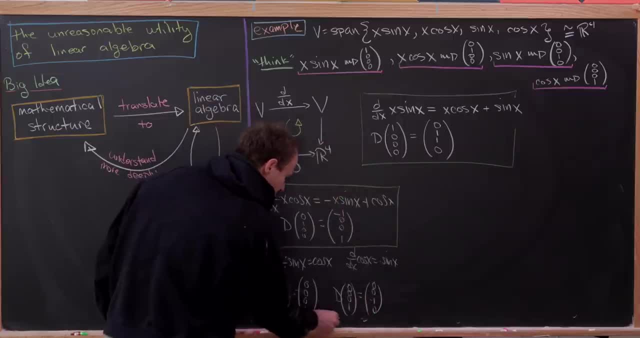 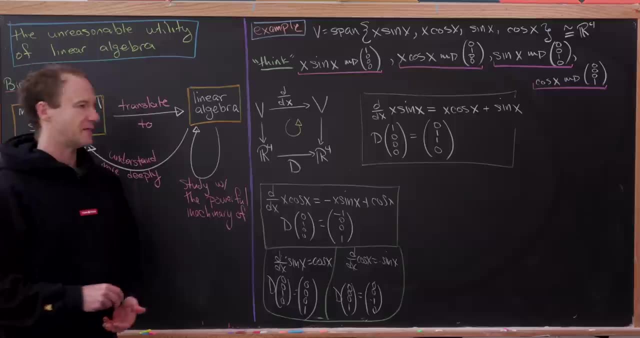 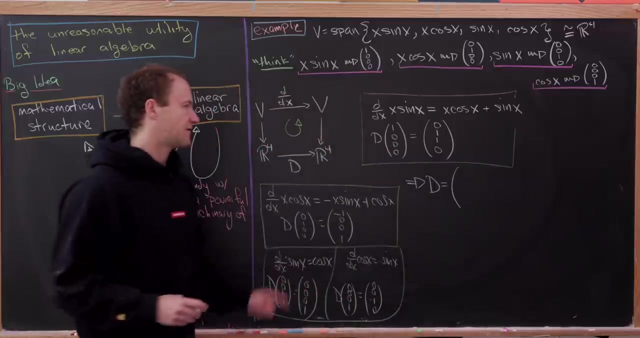 Okay, Great. So there we've got everything we need. We have D acting on all of the standard basis vectors, But that gives us the shape of D, So we can just read this off. So D will be 0, 1, 1, 0.. 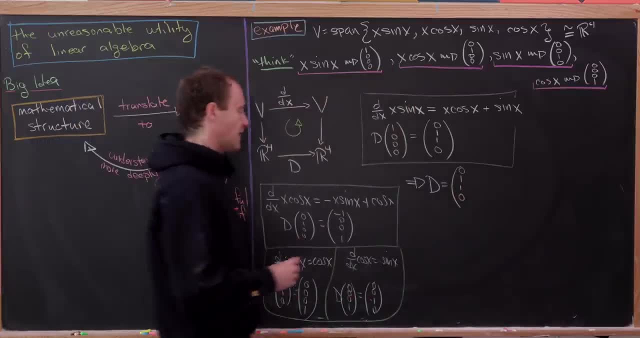 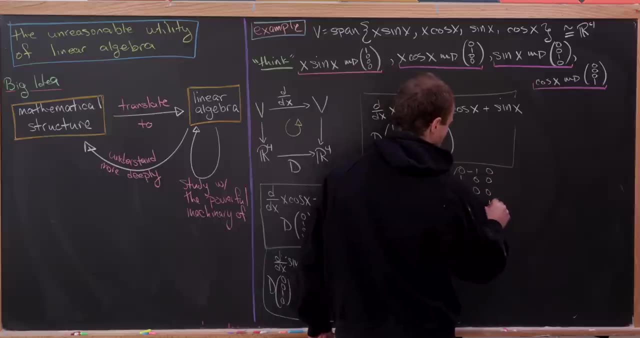 So I'm reading this column wise, And then negative: 1, 0, 0, 1.. And then 0, 0, 0, 1.. And finally 0, 0, minus 1, 0.. 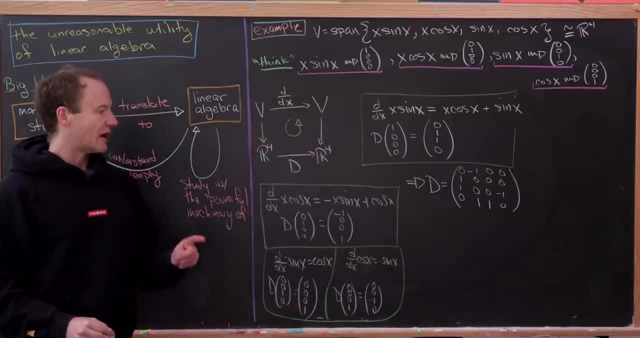 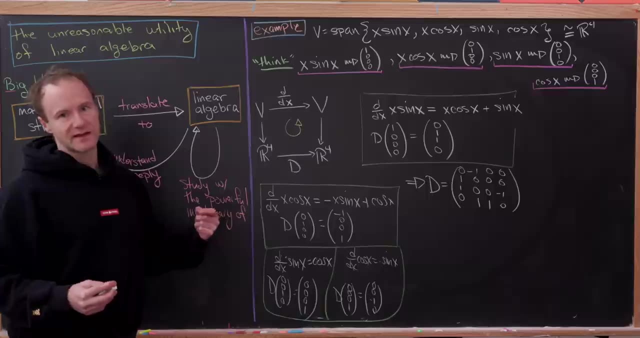 Okay, So there we have it Now as an application. I'd like to take its inverse and think about: well, what's the inverse of the derivative? Well, it's the antiderivative or the indefinite integral, And well, I won't go through the details here. 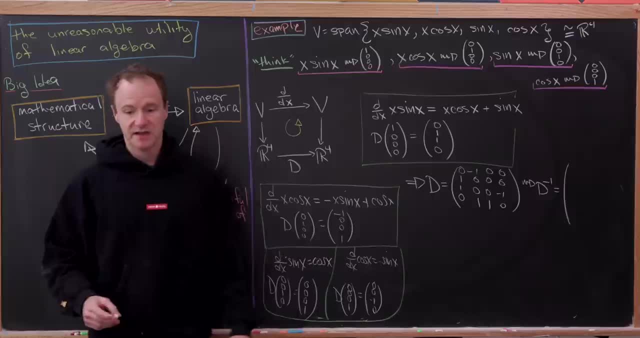 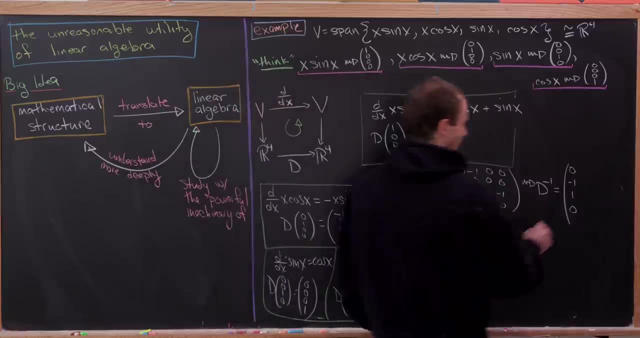 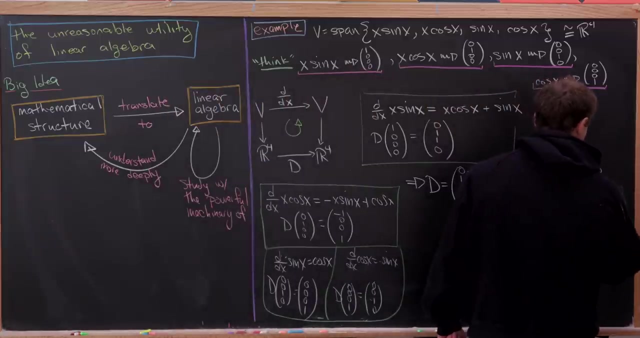 But D inverse can fairly easily be calculated to be 0, negative 1, 1, 0.. That's our first column, And then 1, 0, 0, 1.. That's our second column, And then 0, 0, 0, negative 1.. 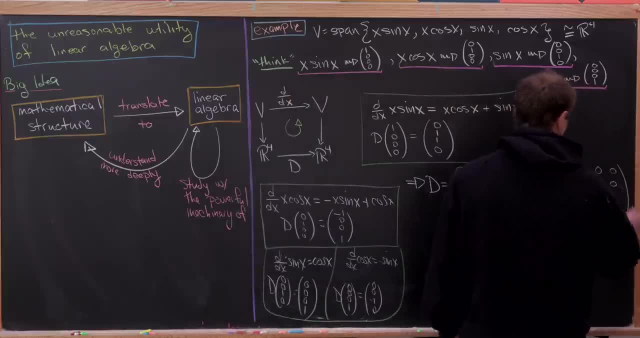 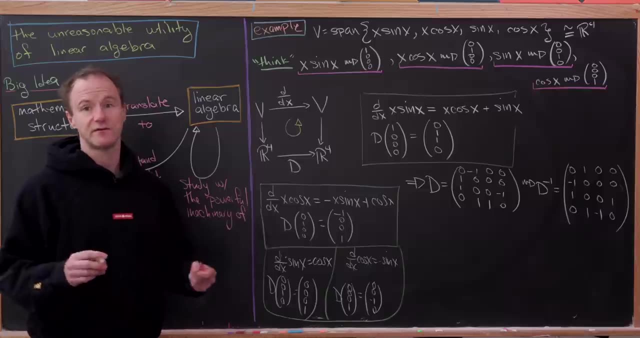 And then finally 0, 0,, 1, 0. Great. So that means if we wanted to do something that would generally be kind of tricky, in fact involve integration by parts, like the integral of x sine, of x Dx. 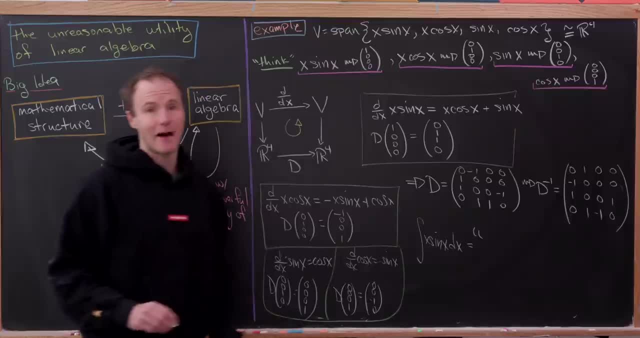 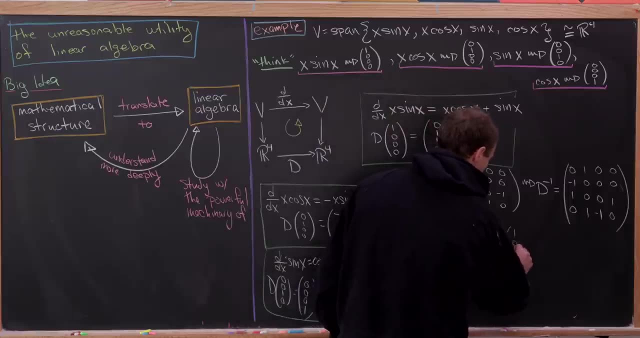 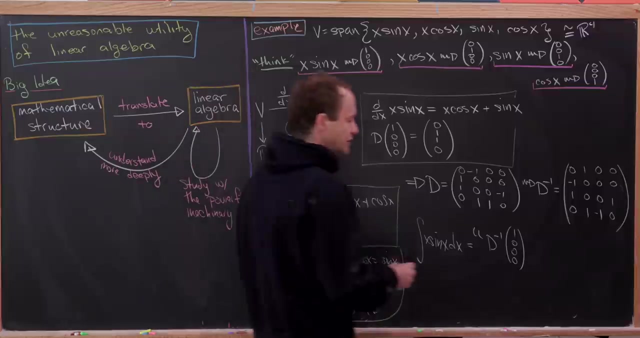 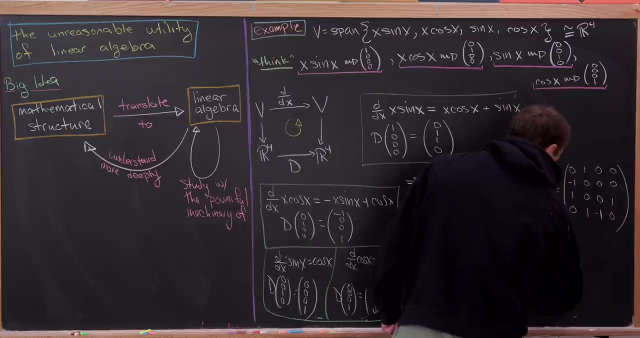 We can instead think of this happening within the matrix vector world. So this should be D inverse of 1, 0, 0. Where D inverse is, well, the matrix that I have up there. So you can do the matrix multiplication and you'll see that this is equal to 0, negative 1, 1, 0. 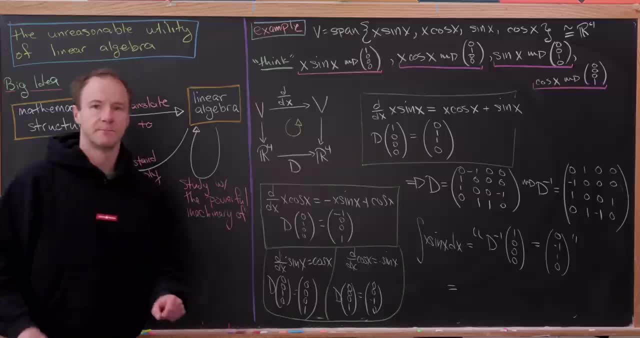 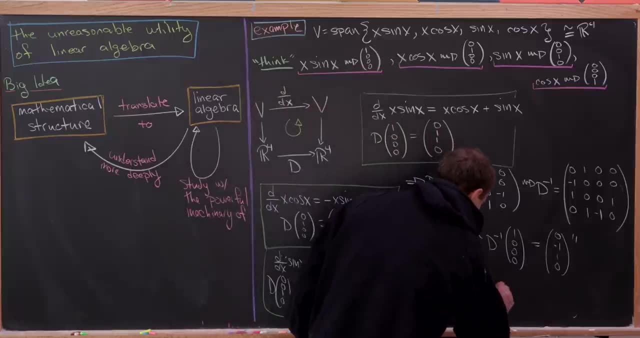 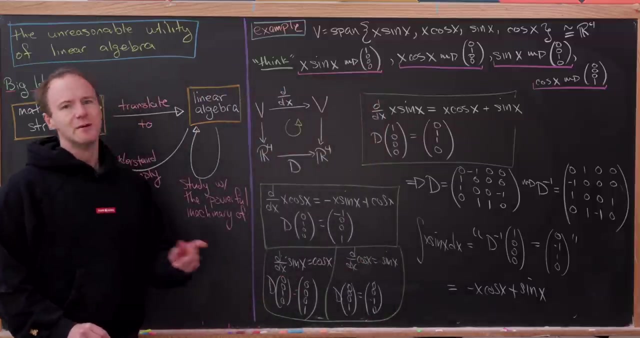 But then putting that back into terms of our sine x, cosine y, Sine x, x, sine x, and so on and so forth, We'll see that we get minus x, cos x, plus sine of x, Which of course we're missing, the plus a constant. 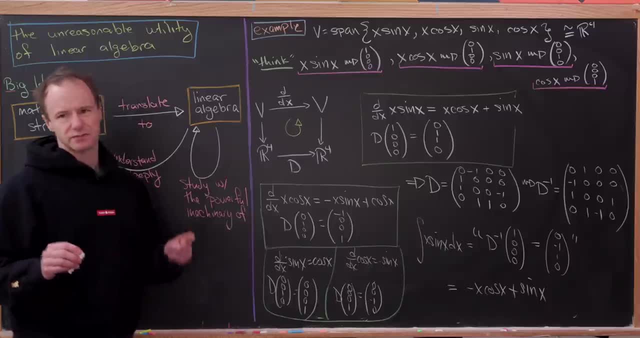 But that's because that's not encoded into this linear algebra setup here. But that is in fact the antiderivative that you would get by doing the integration by parts here. Okay, so let's look at another example. So for our next example, 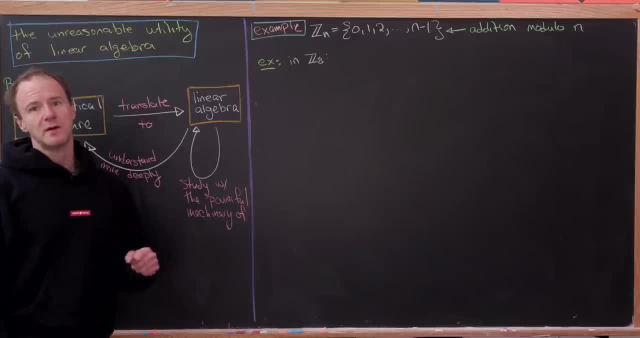 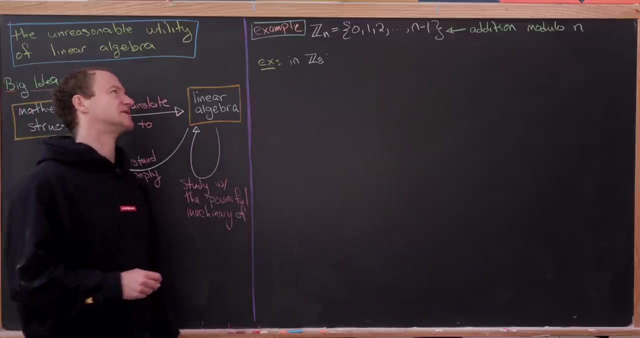 I'll do an example of how a group may be represented in linear algebra via a matrix, And the group that we'll work with here is Zn, Which is the set of equivalence classes modulo n. But we can really think about it just as the numbers 0,, 1,, 2,, all the way up to n minus 1.. 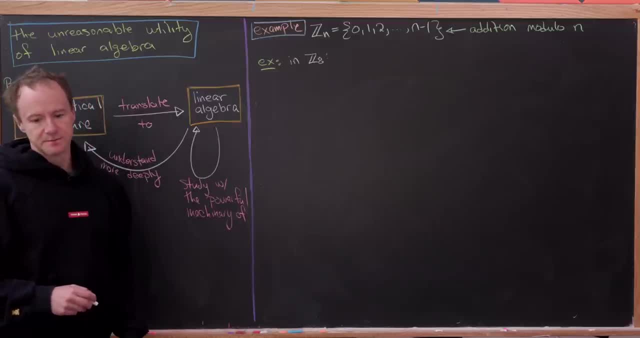 Where addition is done, modulo n, Which means we take the normal sum of two numbers but then divide by n and keep the remainder. In other words, we reduce mod n. So, for example, so that we're all on the same page. 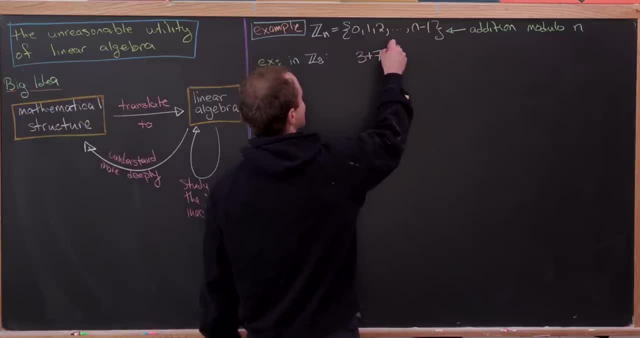 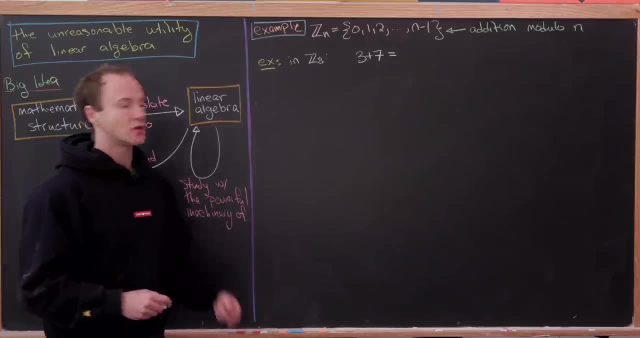 inside of Z8, we have 3 plus 7.. You might think that that's equal to 10.. But if we divide by 8 and keep the remainder, we get the number 2.. That's because the quotient would be 1 and then the remainder would be 2.. 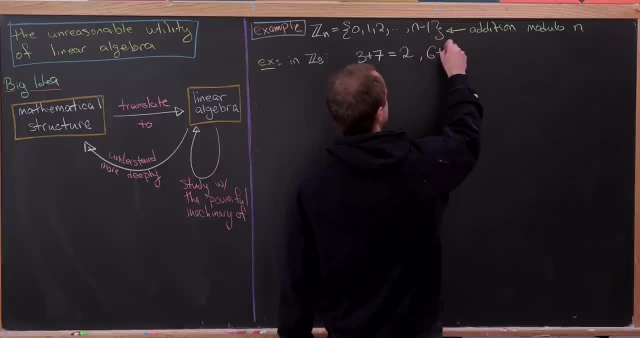 And then, similarly, 6 plus 5,, that looks like 11,, but mod 8 is 3.. And then, finally, if we look at something like 4 plus 4,, well, that's going to be 8, but that's equal 0 mod 8.. 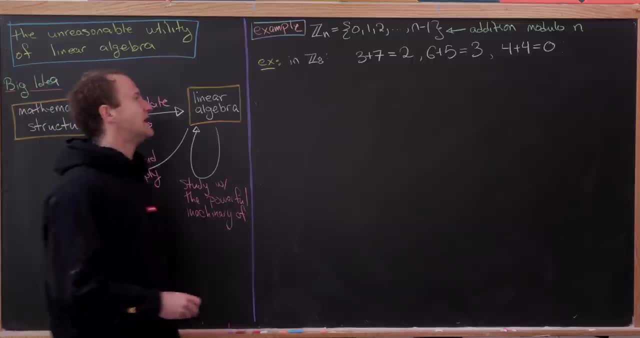 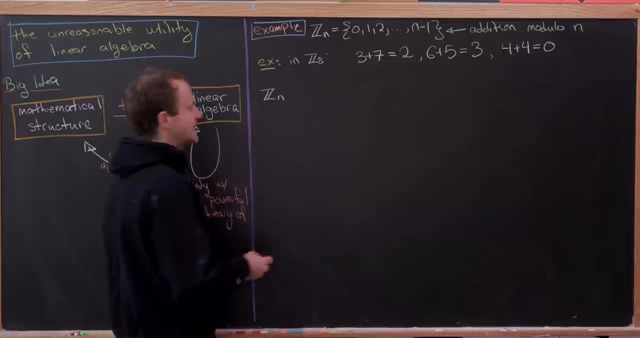 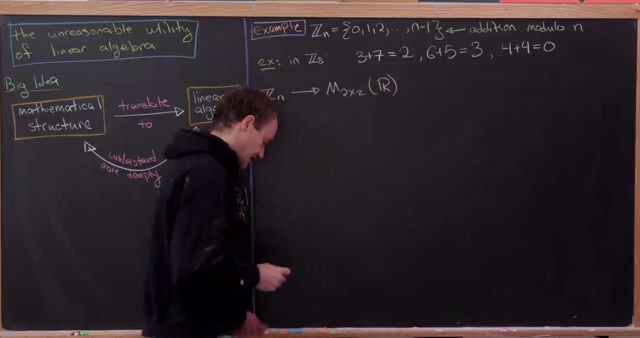 Because it's a multiple of 8.. But now what we'd like to do is somehow take elements of Zn and write them as matrices, And here's how we can do it. So we can in fact write these as 2 by 2 matrices with real entries. 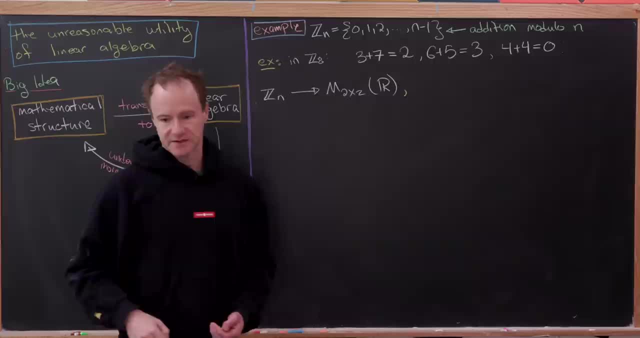 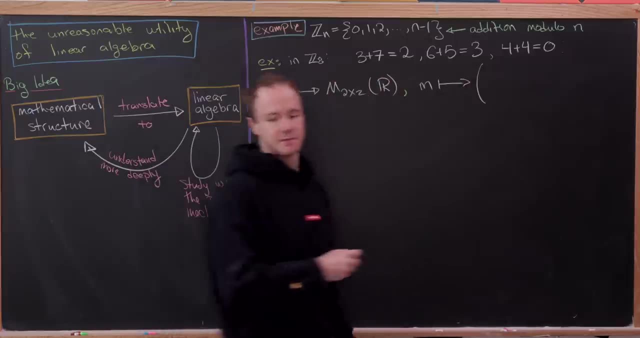 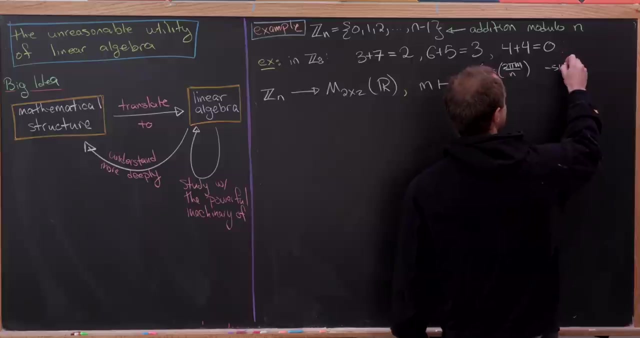 And the assignment goes like this. So we'll take the number m and we'll assign it to the following 2 by 2 matrix, So it'll be cosine of 2 pi m over n and then minus sine of 2 pi m over n. 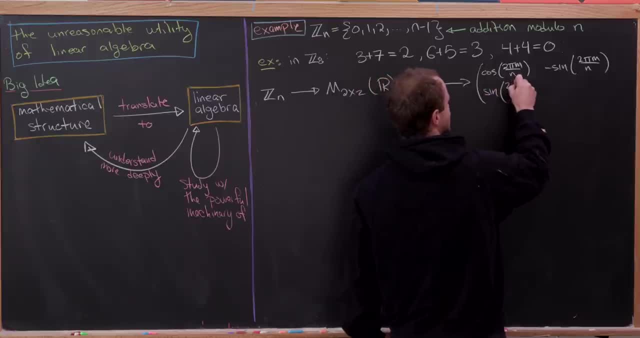 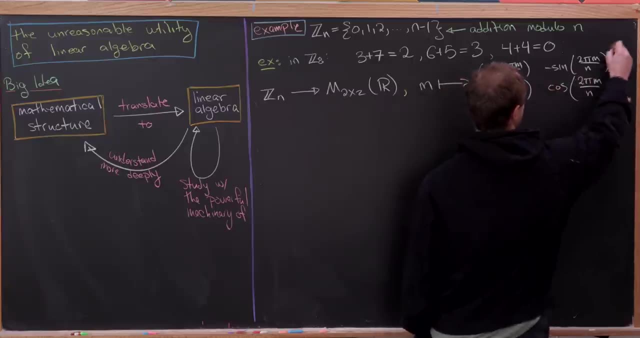 And then down here we'll have sine of 2 pi m over n. And then here we'll have cosine of 2 pi m over n. And then here we'll have cosine of 2 pi m over n. And then here we'll have cosine of 2 pi m over n. 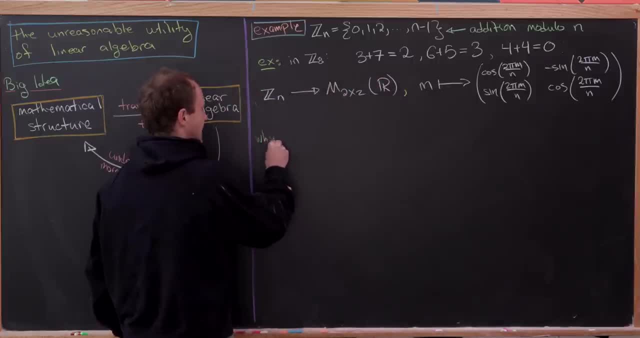 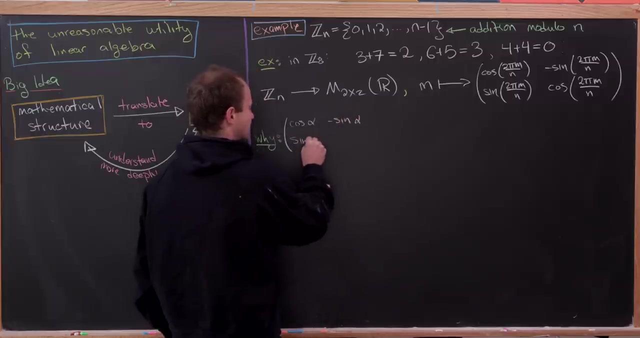 And let's maybe see why this works. And it all comes down to the fact that this really looks like a rotation matrix And in fact we've got this more general formula that if we have a cosine alpha, a minus sine alpha, a sine alpha and a cosine alpha matrix, 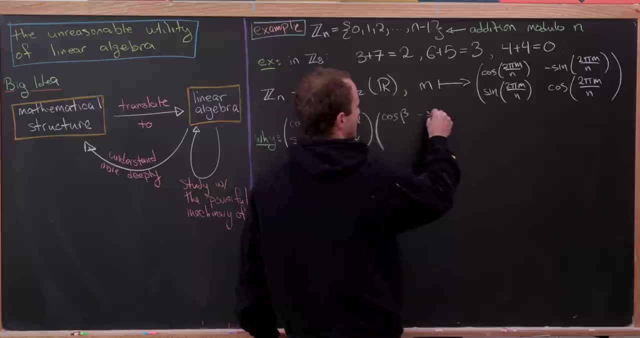 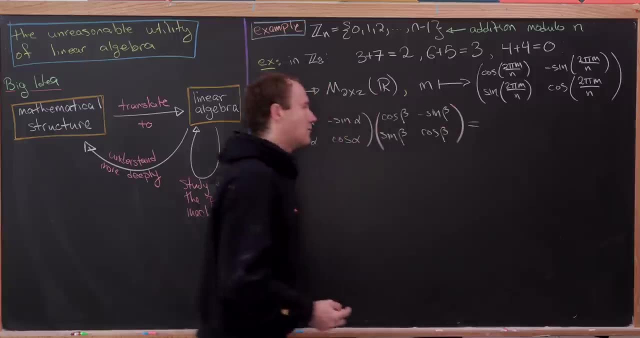 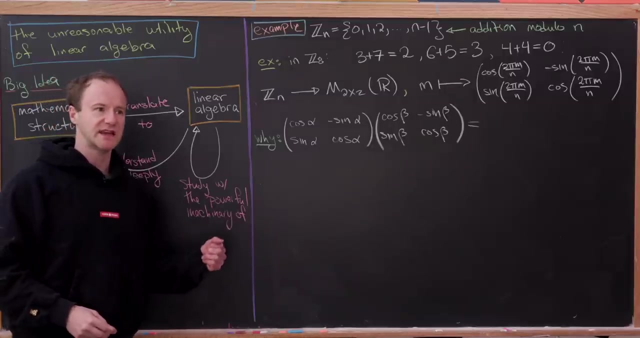 and then a similar cosine beta minus sine beta, and then sine beta and cosine beta matrix. if we multiply these 2 matrices, well, I won't write it out long ways, but what you'll see is that the entries look suspiciously like. 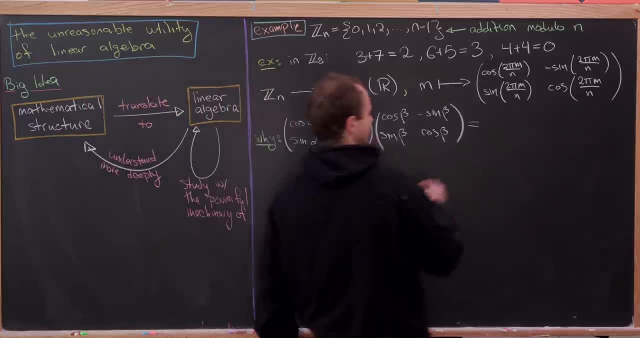 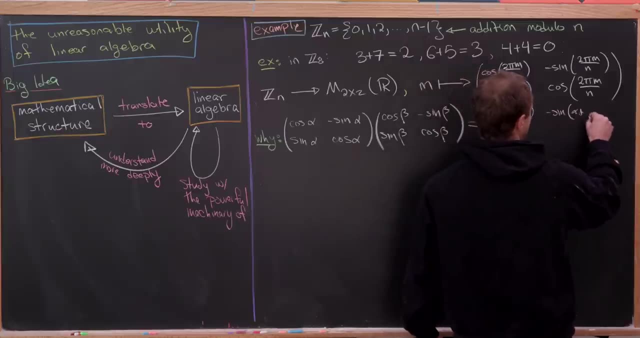 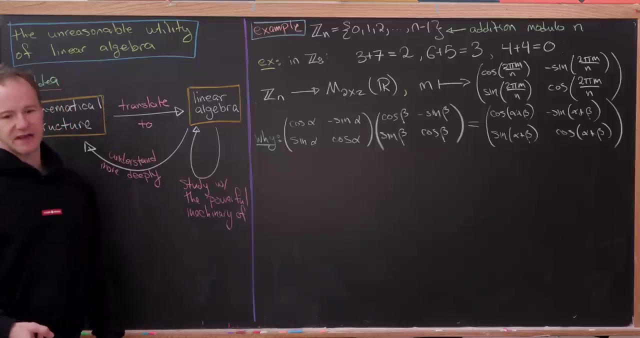 the sum angle formulas for sine and cosine, And that gives us the following matrix: Cosine of alpha plus beta minus sine of alpha plus beta. And then here we have sine of alpha plus beta and cosine of alpha plus beta. So in fact we've turned addition into matrix multiplication. 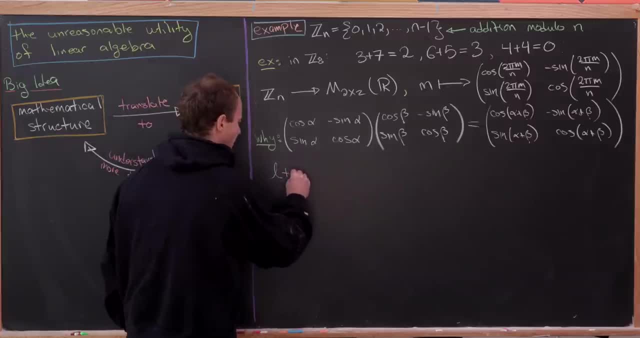 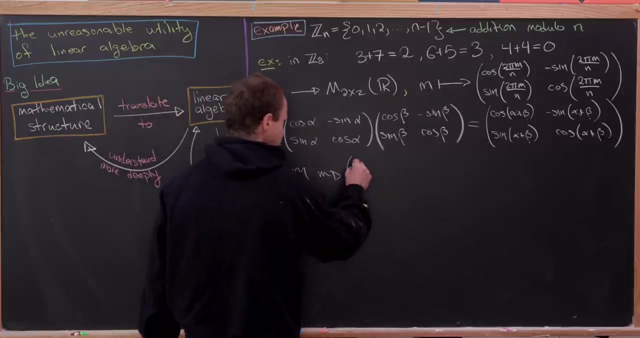 So let's see If we have l plus m happening inside of z n. well, that should look like well, this matrix multiplication with, inside of m, 2 by 2 r. So let's check that it works. So I'm just going to copy these things down. 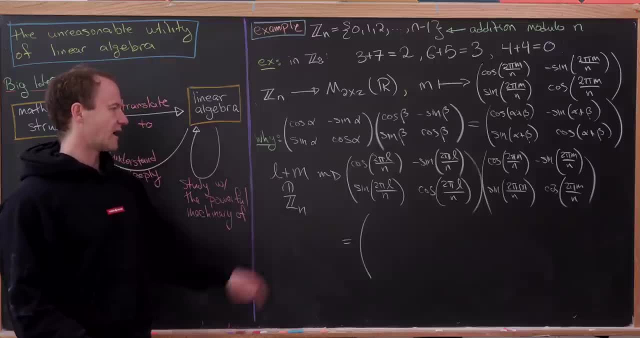 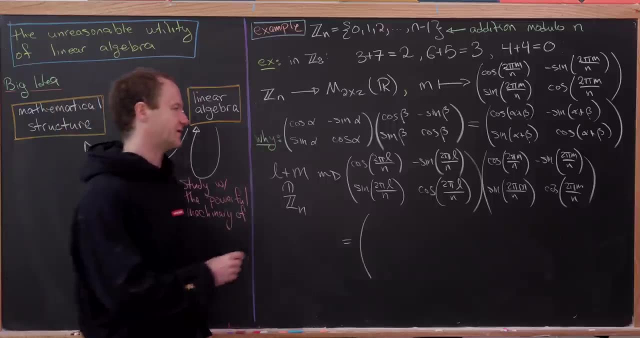 Okay, so there's copying down the matrix associated to l and the matrix associated to m, But then, by this sum rule that we had for the cosine and sine function, that's going to give us, in this top entry, the cosine of 2 pi. 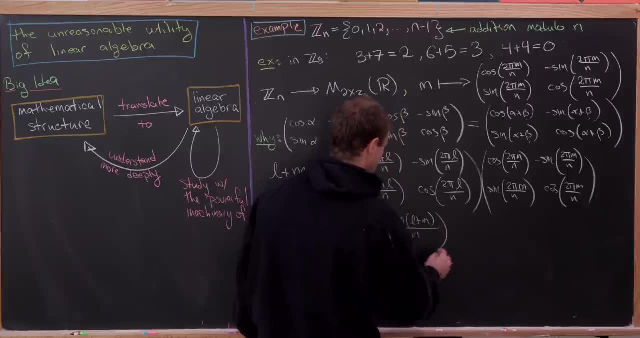 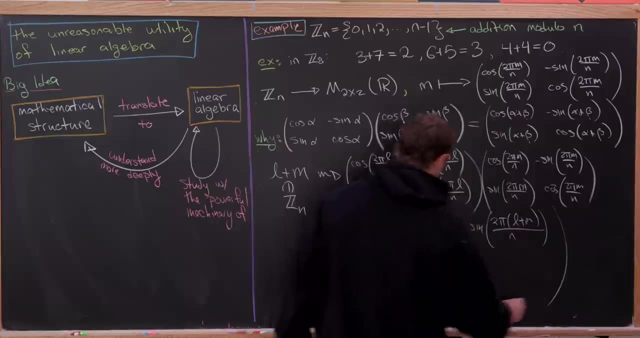 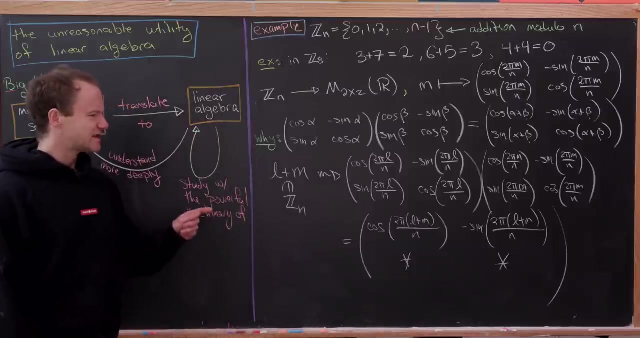 and then l plus m over n, And then here we'll have minus sine of 2 pi and then l plus m over n, And then I'll just put stars down here for similar entries in the lower bit. But let's notice that sine and cosine are both 2 pi periodic. 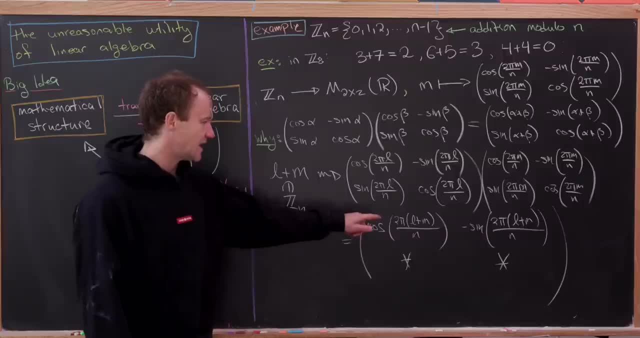 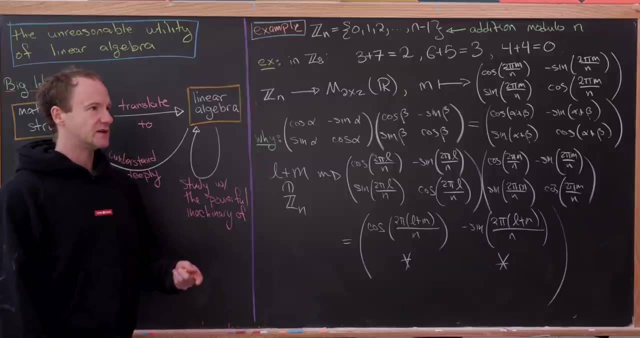 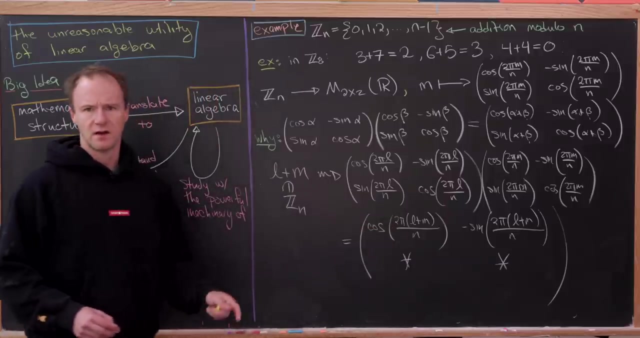 So that 2 pi periodicity here means that this addition is really working modulo n, Because we could divide by n and we'll simply get a multiple of 2 pi out of this right here. But you know, like I said, that's exactly the same. 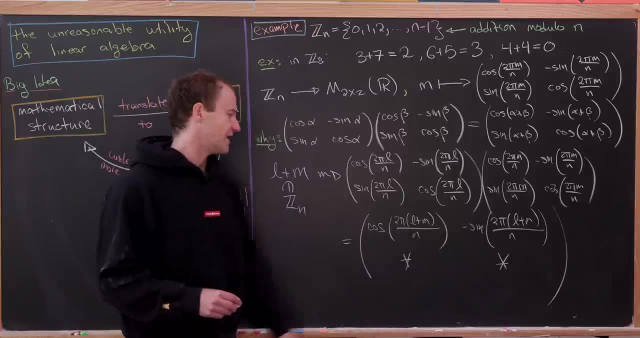 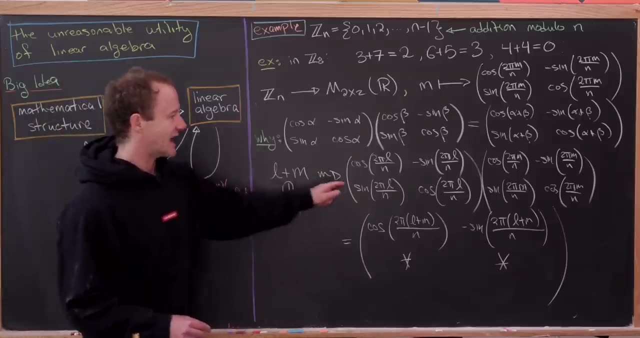 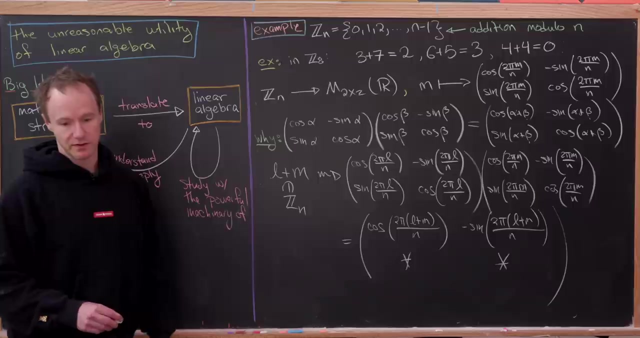 as doing addition modulo n within this cosine function, And so that's allowed us to represent this addition modulo n as matrix multiplication in this, you know, set of matrices with entries in the real numbers. So just as a broader take, this is an example of a group representation. 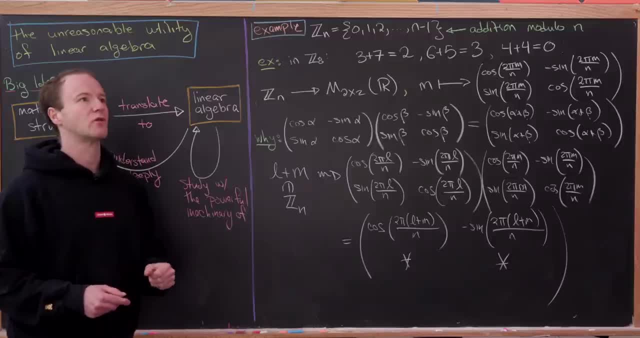 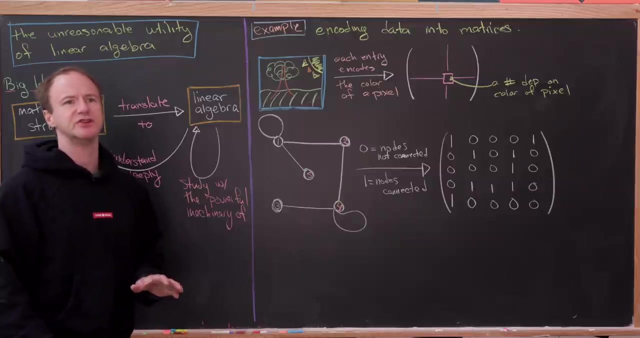 And the representation of groups is like a really important way to study. you know groups in general. Okay, so let's end with one more kind of hint towards an application. Here's another brief glimpse into how linear algebra is used in kind of the modern world of data science and machine learning. 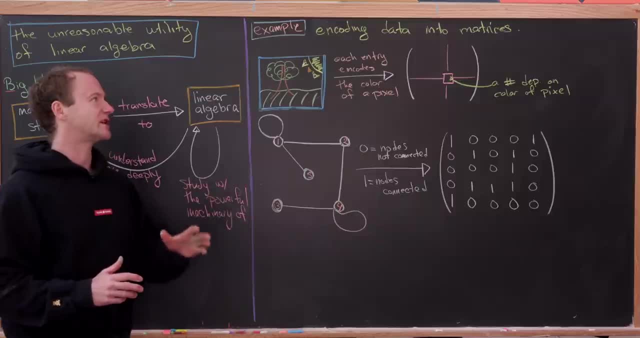 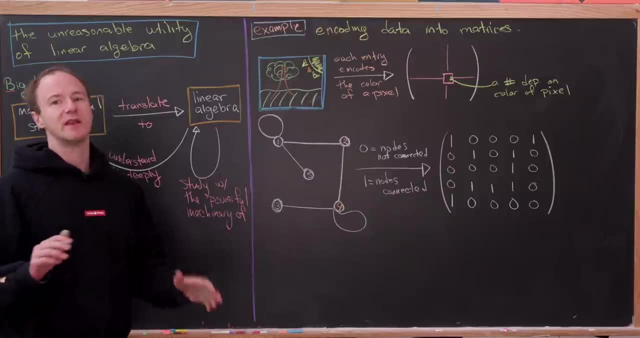 And so broadly, we want to think about ways to encode data into matrices. And then, once that data is encoded into matrices, well, you might do a number of things with it. Perhaps you would do a so-called singular value decomposition, or maybe you do some sort of other matrix factorization rule. 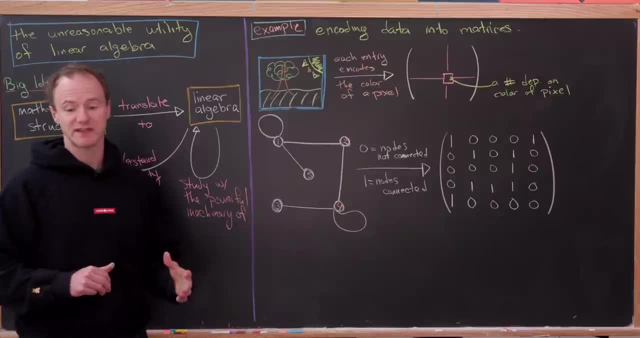 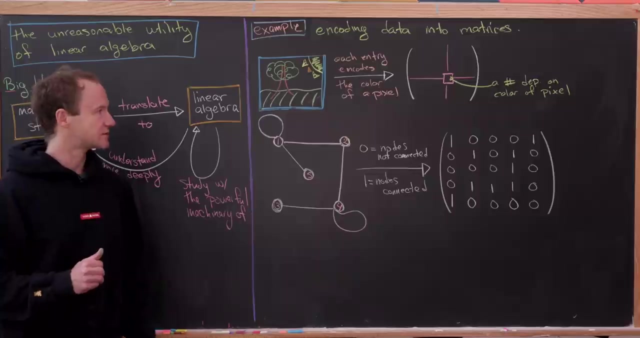 And which one you choose will depend on exactly what parts of the data you'd like to highlight. So this is like really kind of a big subject at the moment, so I'm not going to really go into it that deeply. It would take many, many hours. 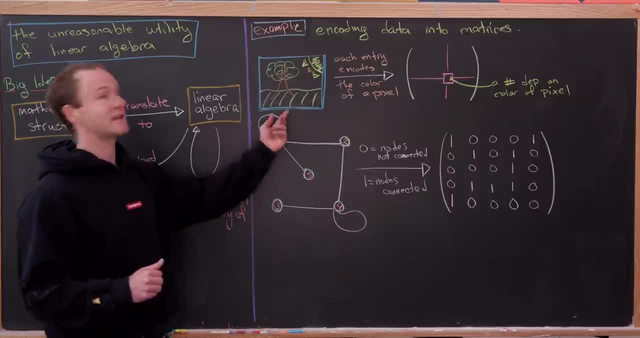 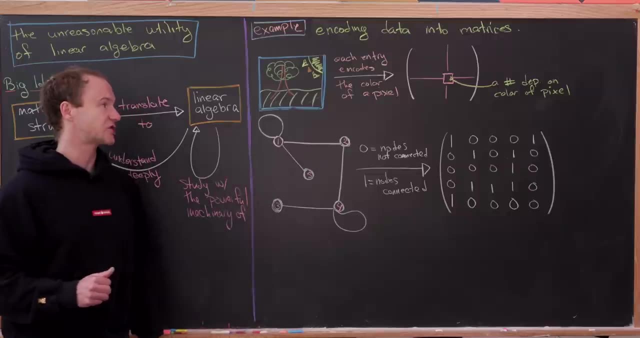 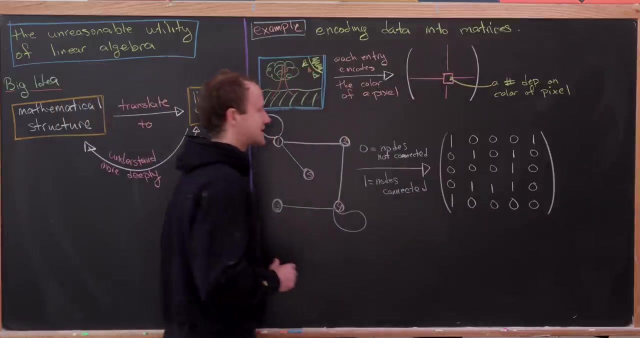 But just really briefly. you could like take a picture like this wonderful picture that I've drawn, and you could encode each pixel of this picture into a matrix via its color. So, in other words, we've got this matrix over here and the size of the matrix is well, it depends on the number of pixels. 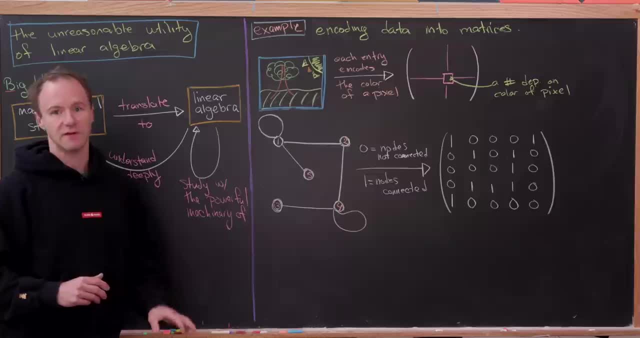 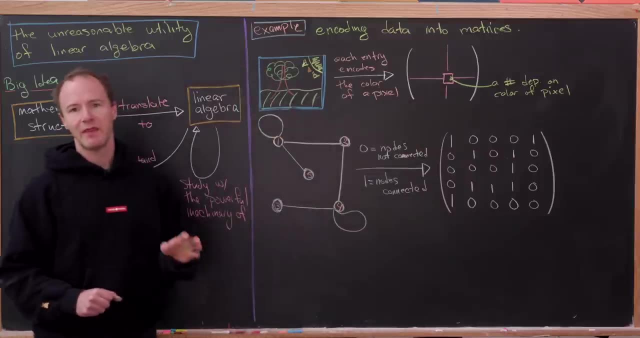 kind of in the horizontal and vertical direction of this picture And you go to a certain interval and there's an entry of this matrix and there's going to be a number in there And that number is going to depend on the color of the pixel, like I said. 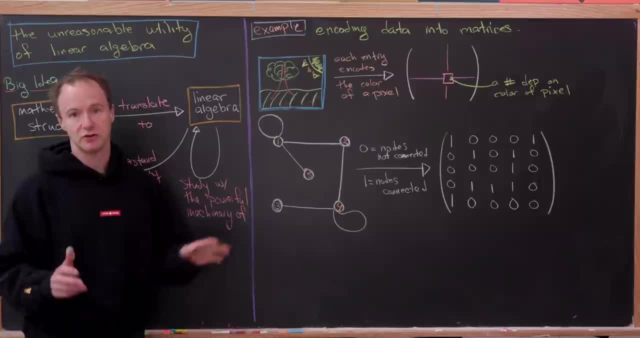 And so that'll encode this picture into you know, an array or a matrix, if you want to think about it using linear algebra terminology. Another thing you could look at is a network or a graph, And so in a graph you've got so-called vertices or nodes. 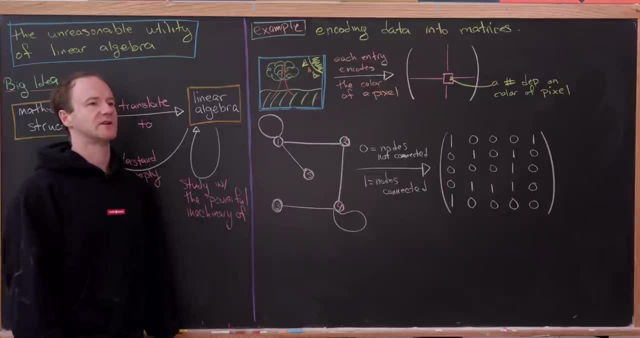 and you have edges which are connections between the vertices or nodes, And so graph theory or maybe the study of these networks are kind of one and the same And they have a lot of like really interesting applications into how the web works at the moment. 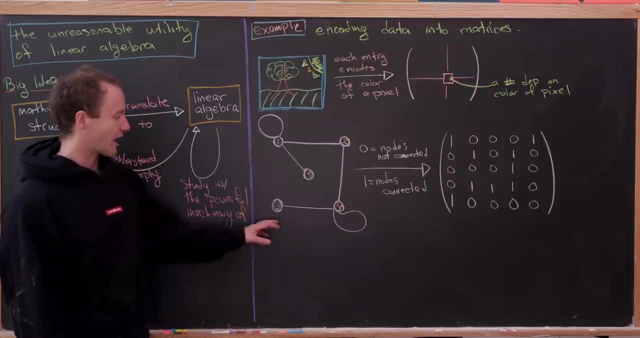 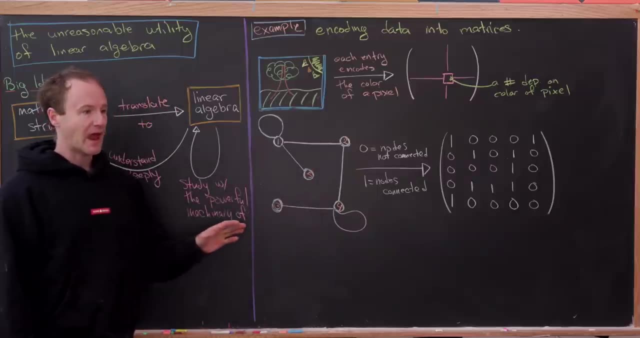 So here's a really simple example. So we've got a graph with five vertices, So one, two, three, four, five is how I've labeled them- And we could encode this graph into something called an adjacency matrix, And in an adjacency matrix you get zeros if nodes are not connected. 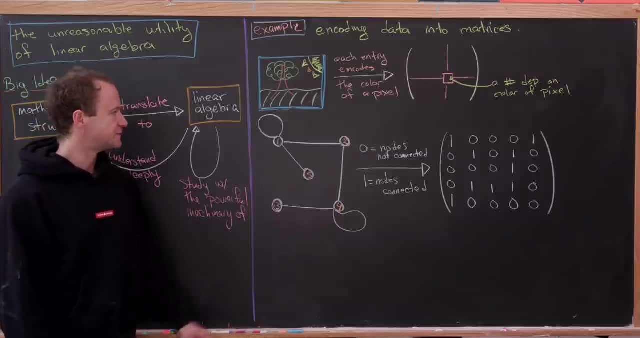 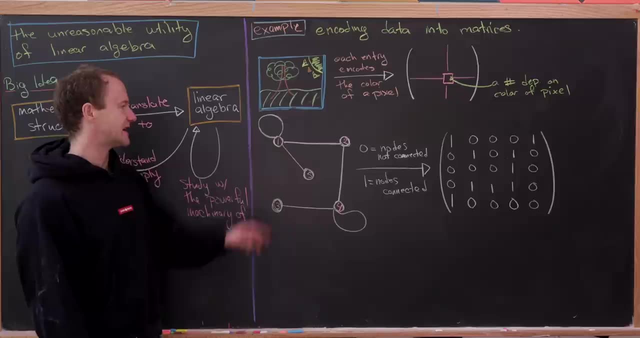 or you get ones, if nodes are connected. So let's notice that one has an edge from itself to itself and an edge to five. So that means one is connected to itself and to five. So that means in this first column, which is the column representing this first node one. 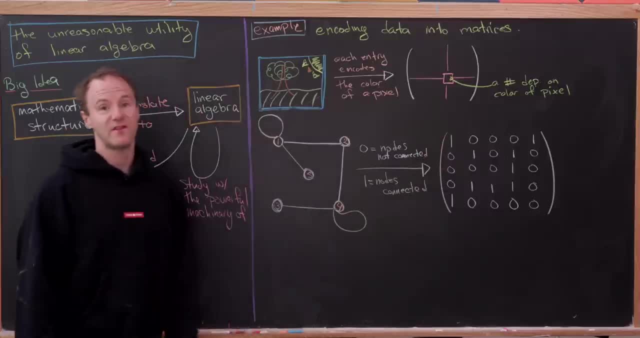 you've got a one in the first entry and one in the fifth entry, but zeros everywhere else is So that represents the connection to itself and to five, And then for all of the other nodes you have similar ways of building those columns. 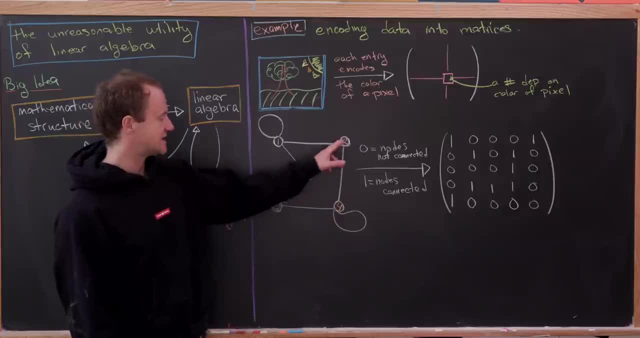 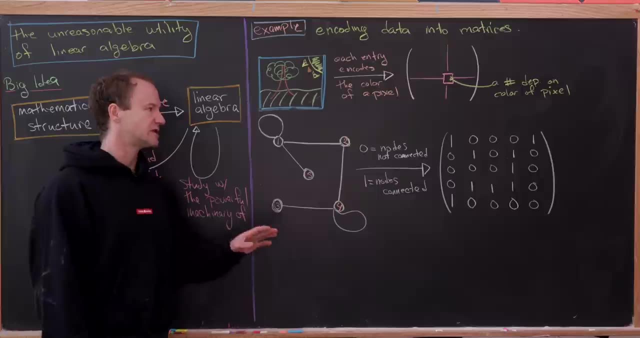 So, for example, the fourth node is connected to the second, the third and itself. So if you go over here to this fourth column, you see that you have zeros in the first and the fifth entry, but one everywhere else. Okay, so there you have it. 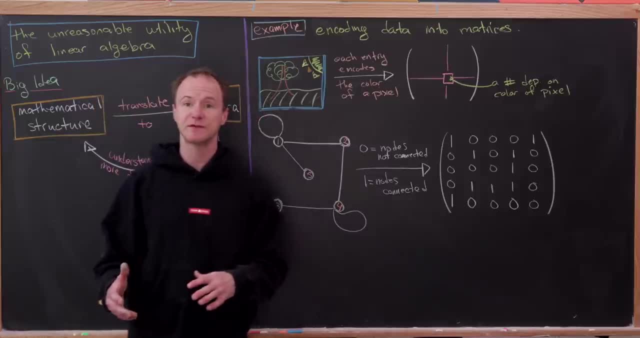 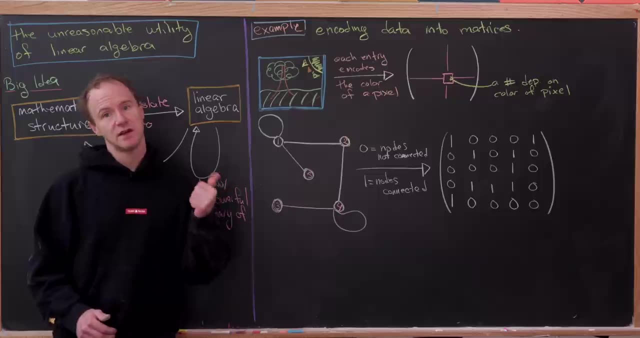 Three examples of how linear algebra is suited and super useful in studying ideas from mathematics And in fact, these areas of mathematics that we've looked at, you know: differential calculus, and then group theory, and then you know, maybe data science. 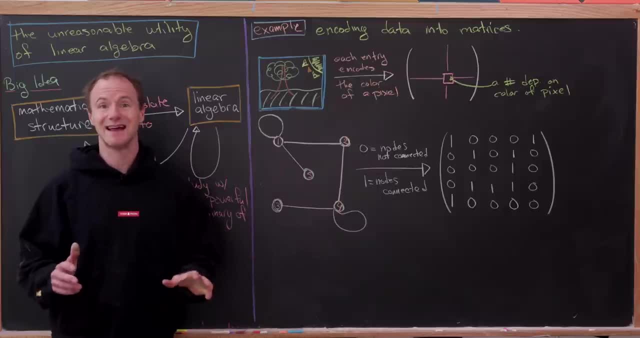 seem to be pretty disconnected in their own right. So I think it's nice that linear algebra forms kind of a certain universal language for studying all of them. So maybe post in the comments your favorite application of linear algebra And thanks for sticking around. That's a good place to stop.